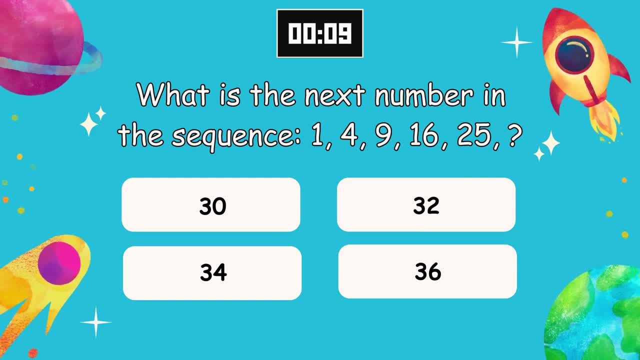 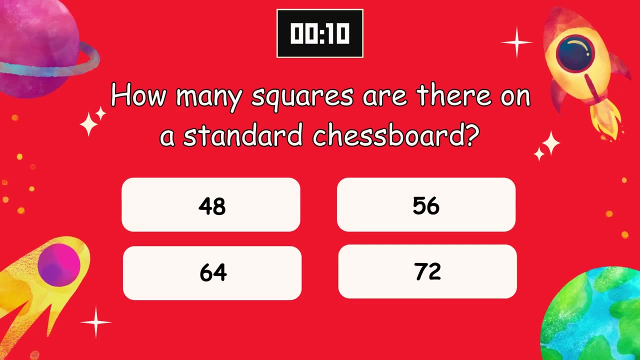 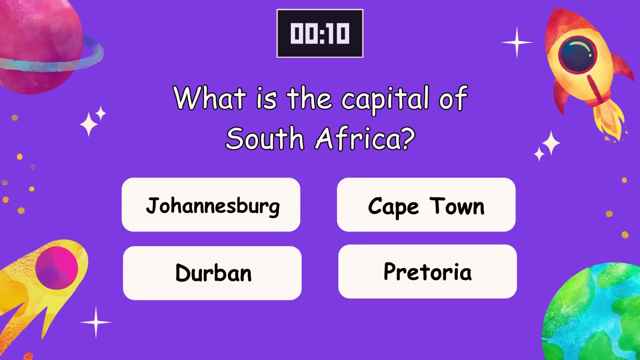 what is the next number in the sequence 1, 4, 9, 16, 25, 30, 32, 34, 36? correct answer is 36. how many squares are there on a standard chessboard? 48, 56, 64, 72? correct answer is 64. what is the capital of south africa? johannesburg, cape town, durban, pretoria. 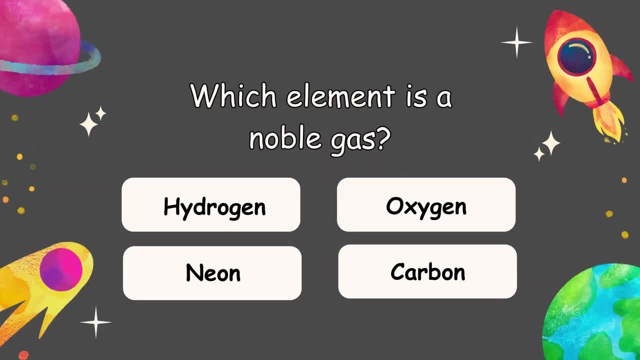 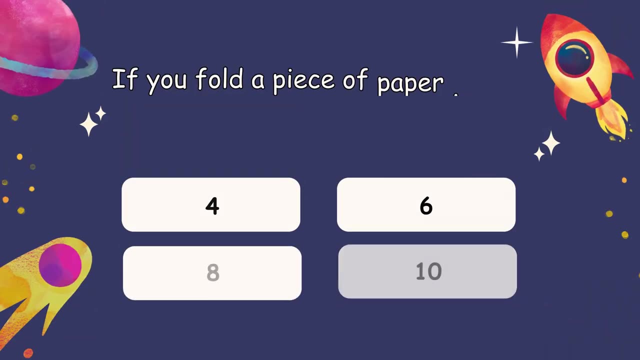 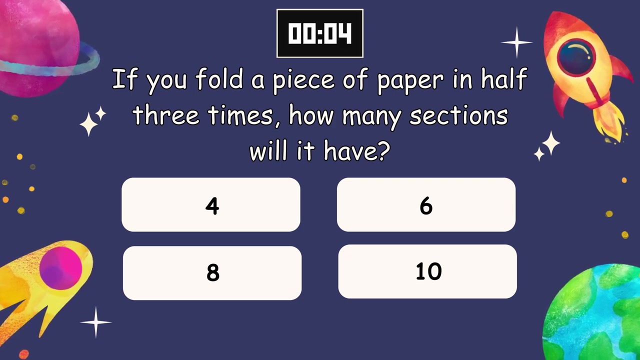 correct answer is pretoria. which element is a noble gas? hydrogen oxygen, neon or carbon? correct answer is neon. if you fold a piece of paper in half, three times, how many sections will it have? four, six, eight, ten. what is the missing number in the sequence? 2, 5, 16, 25, 24, 36, 24, 36, 64, 37, 48. 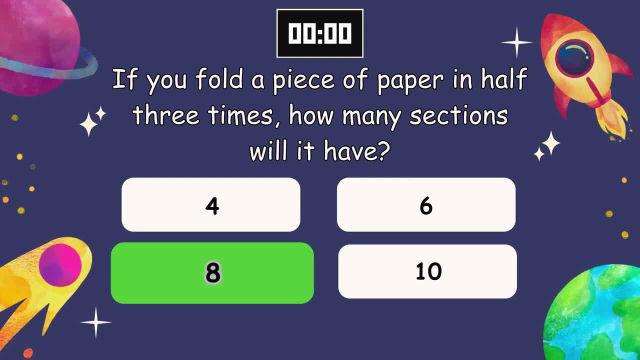 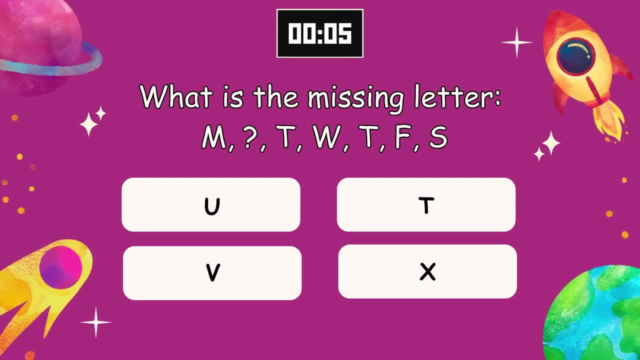 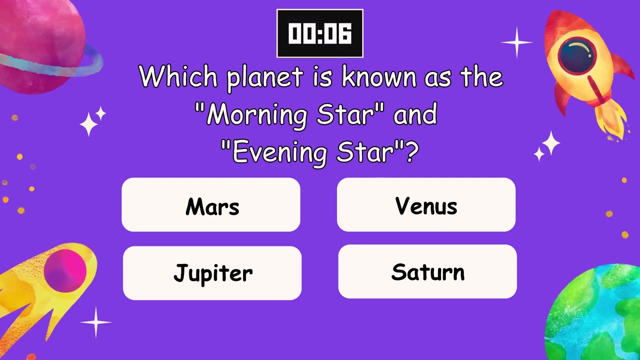 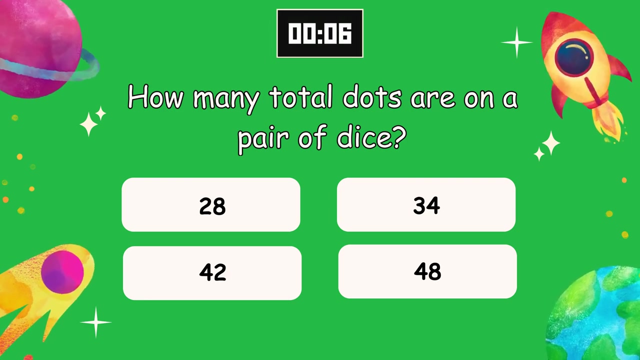 correct answer is eight. what is the missing letter? m, t, w, t, f, s, u, t, v, x? correct answer is t. which planet is known as the morning star and evening star? mars, venus, jupiter, saturn? volatility: correct answer is eight. what is the missing number in the sequence 2? 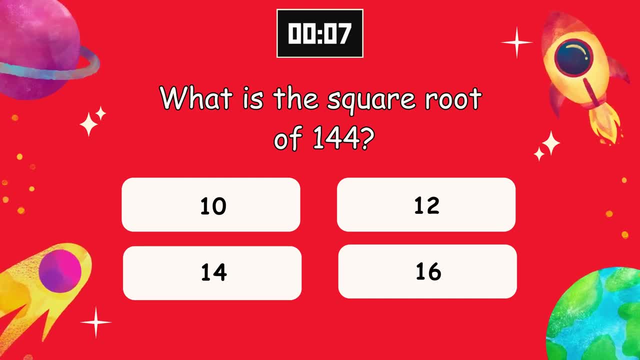 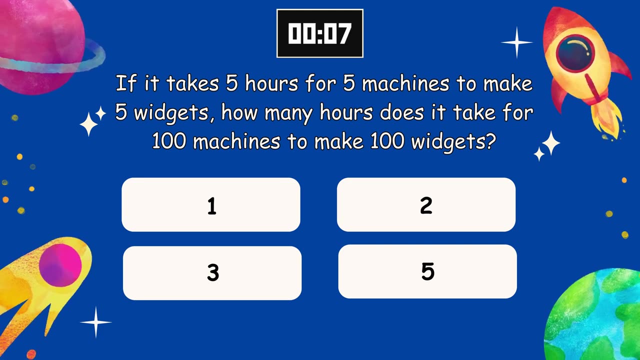 six knight også t nine 24수. correct answer is q. sorry, Correct answer is 12.. If it takes five hours for five machines to make five widgets, how many hours does it take for 100 machines to make 100 widgets? Correct answer is 5.. 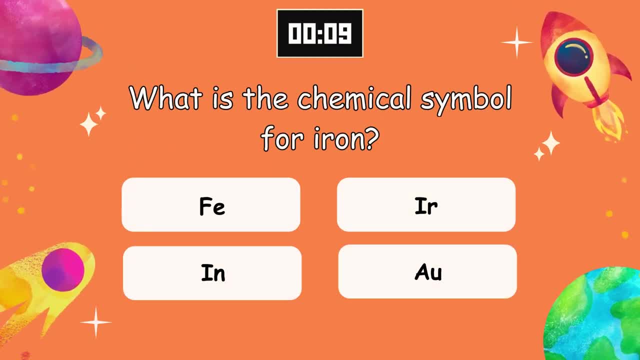 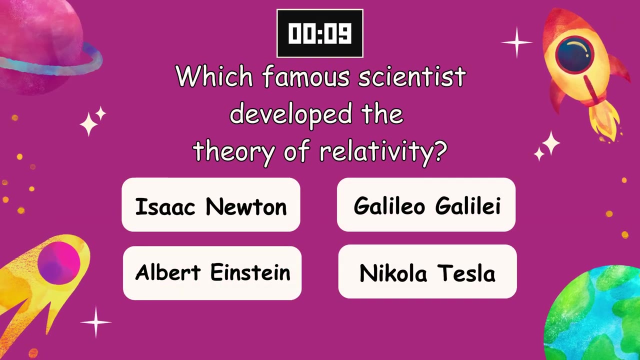 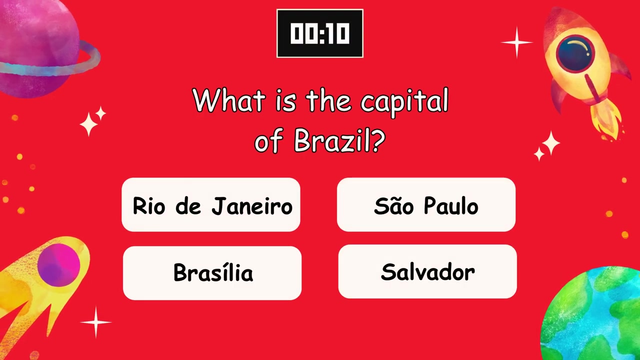 What is the chemical symbol for iron? Correct answer is 5.. Which famous scientist developed the theory of relativity? Isaac Newton, Galileo Galilei, Albert Einstein, Nikola Tesla? Correct answer is Albert Einstein. What is the capital of Brazil? 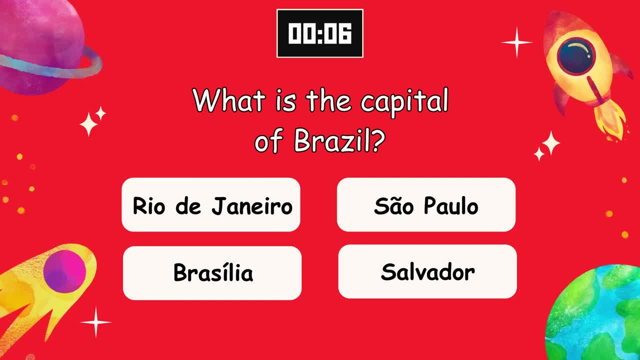 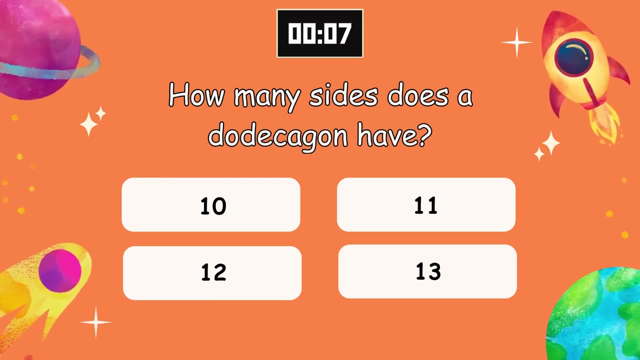 Rio de Janeiro, Sao Paulo, Brasilia, Salvador. Correct answer is Brasilia. How many sides does a dodecagon have? 10,, 11,, 12,, 13.. Correct answer is 12.. What is the sum of the interior angles of a hexagon? 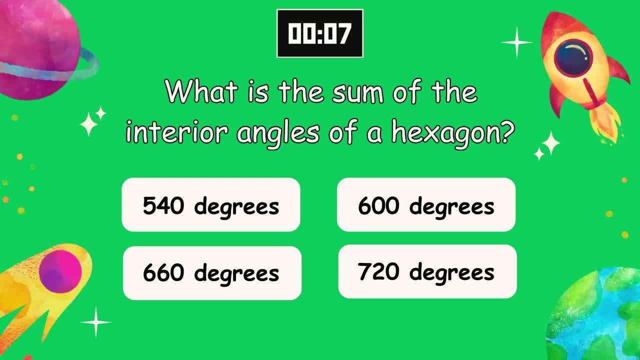 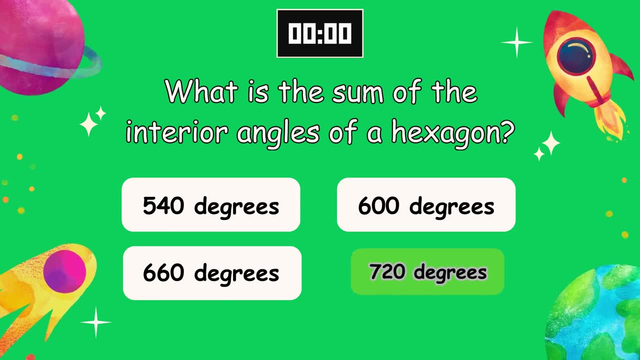 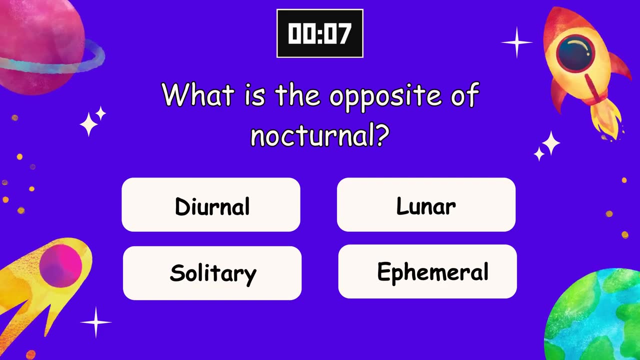 540 degrees, 600 degrees, 660 degrees, 720 degrees? Correct answer is 720 degrees. What is the opposite of nocturnal, Diurnal, lunar, solitary, ephemeral? Correct answer is diurnal. Which element has the atomic number 1?? 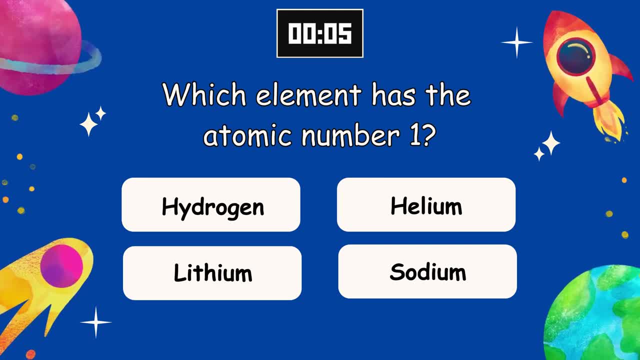 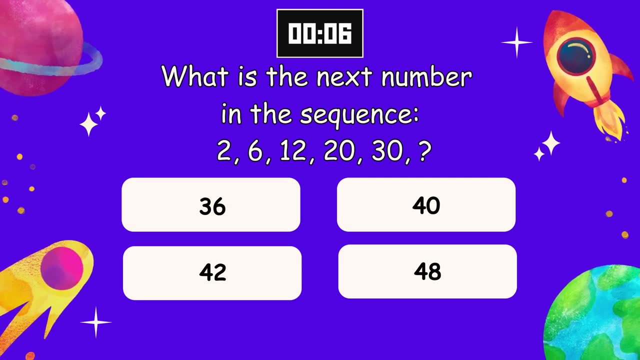 Hydrogen, Hydrogen, Helium, lithium, sodium. Correct answer is hydrogen. What is the next number in the sequence? 2, 6, 12, 20, 30, 36,, 40,, 42,, 48.? 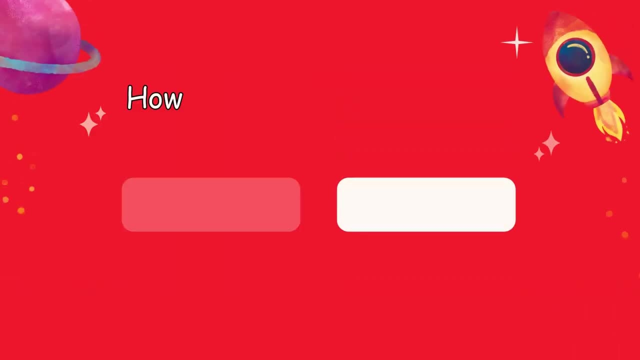 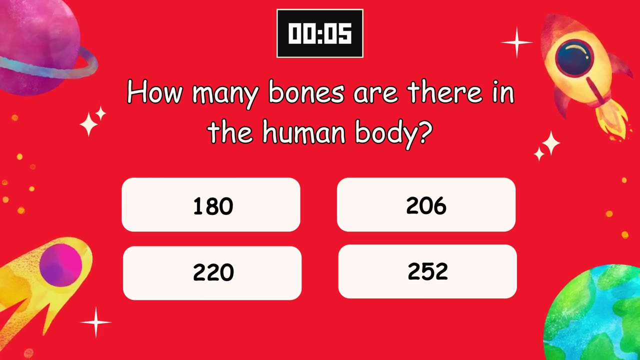 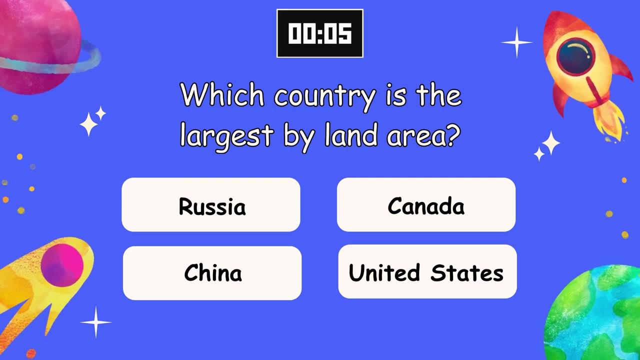 Correct answer is 42.. How many bones are there in the human body? 180.. 240.. 206, 220, 252.. Correct answer is 206.. Which country is the largest by land area? Russia, Canada, China, United States. 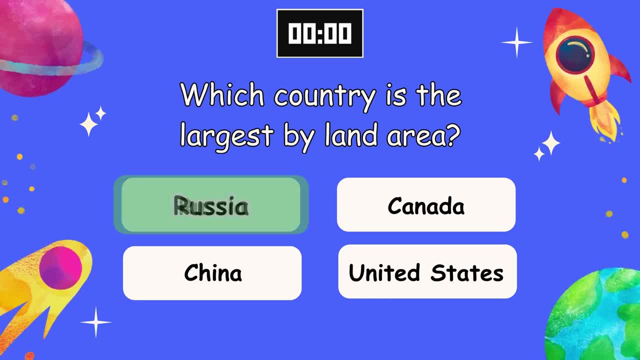 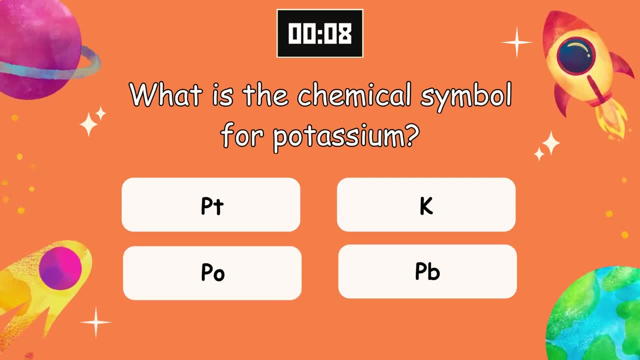 Correct answer is Russia. What is the chemical symbol for potassium? Why is it called potassium? The answer is uncertainty, an absence of vibration on an atom. What makes you think that the bacteria are living in this matter? The answer is volcanic activity. 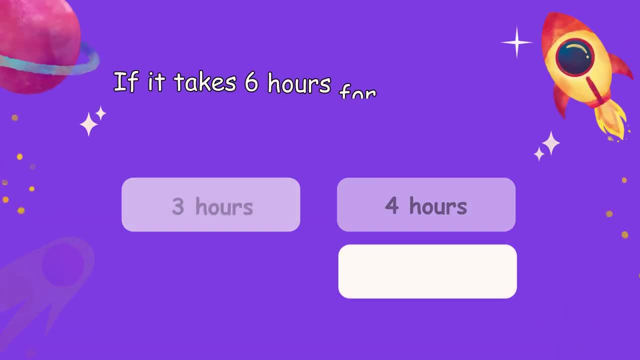 What is the name of the biome? C a, a a, c a c, c a c a c, an a a, a, a a a K? The correct answer is K. 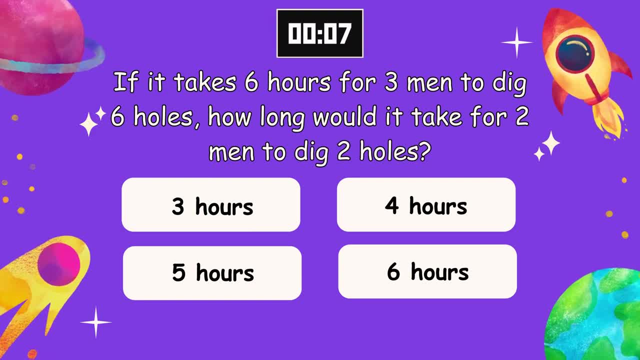 If it takes 6 hours for 3 men to dig 6 holes, how long would it take for 2 men to dig 2 holes? 3 hours, 4 hours, 5 hours, 6 hours, 5 hours. 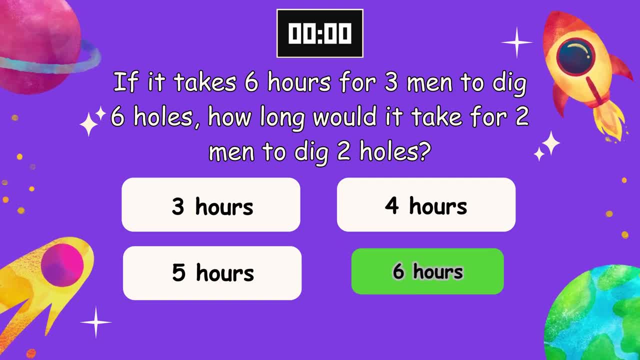 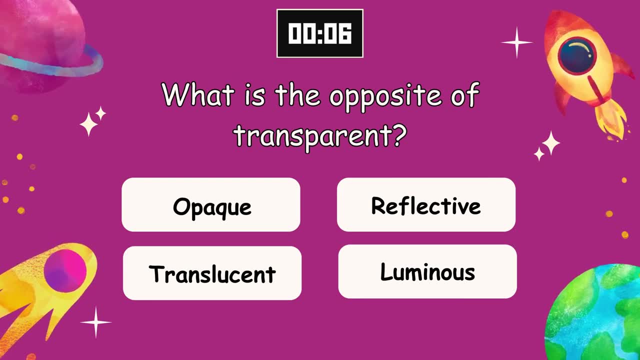 5 hours, 6 hours, 6 hours, 6 hours, 7 hours, 8 hours, 7 hours. Opaque, Reflective, Translucent, Luminous. Correct answer is Opaque. How many strings does a violin typically have? 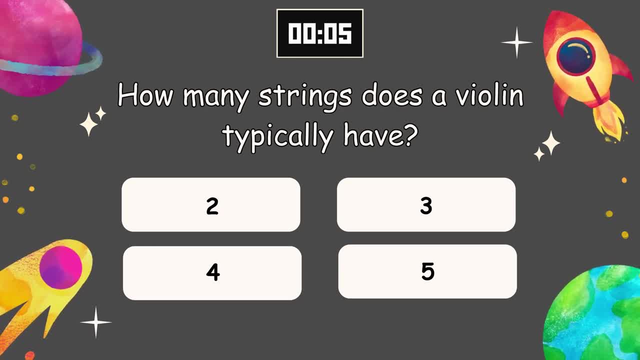 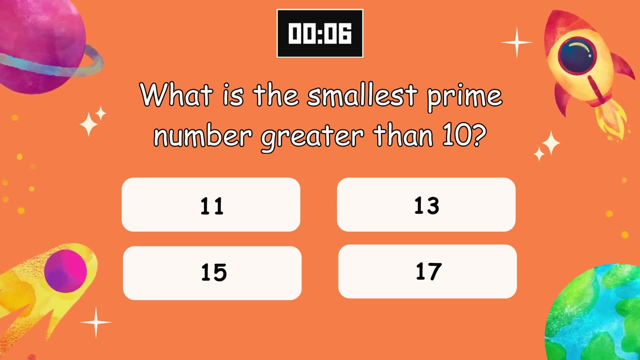 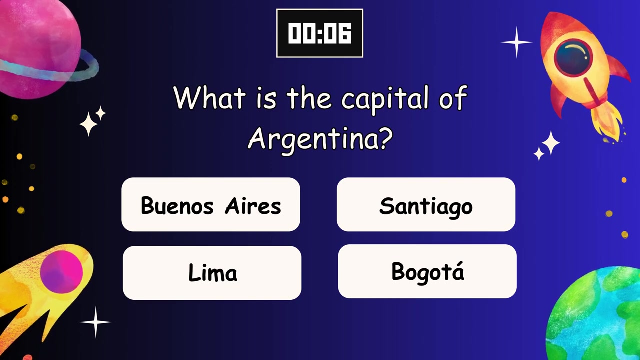 2,, 3,, 4, 5? Correct answer is 4. What is the smallest prime number greater than 10? 11,, 13,, 15,, 17? Correct answer is 11. What is the capital of Argentina? Buenos, Aires, Santiago, Lima, Bogota. 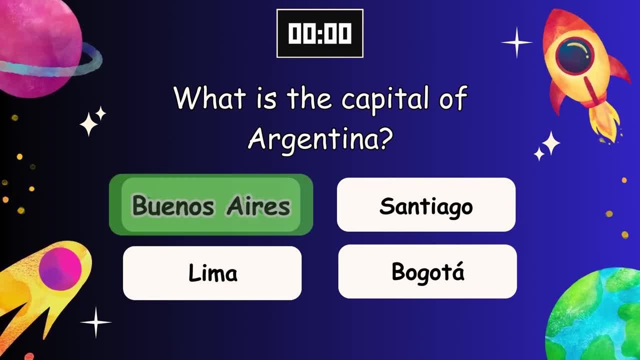 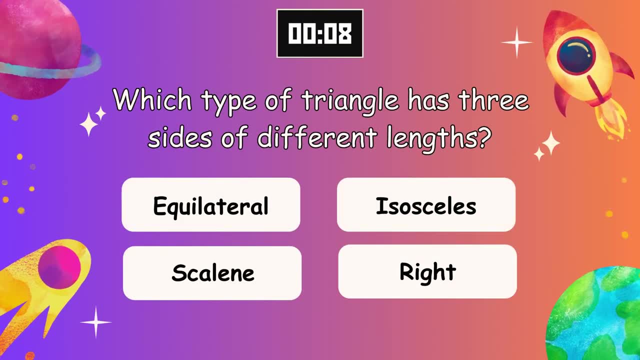 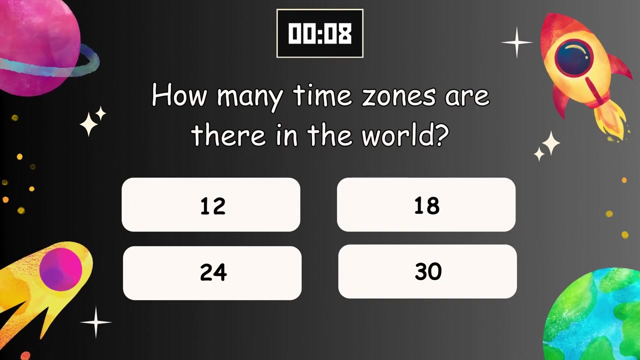 Correct answer is Buenos Aires. Which type of triangle has three sides of different lengths? Equilateral triangle, Isosceles triangle, Scaling triangle, Right triangle. Correct answer is scaling triangle. How many time zones are there in the world? 12,, 18,, 24,, 30. 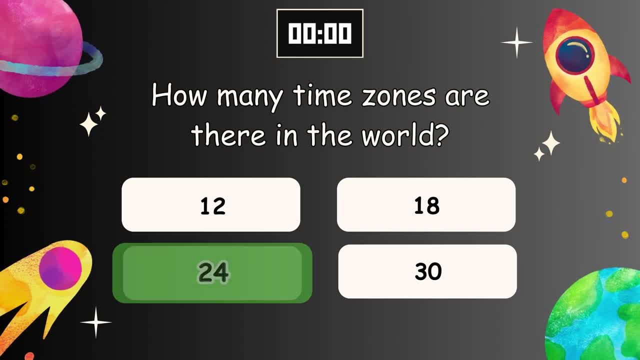 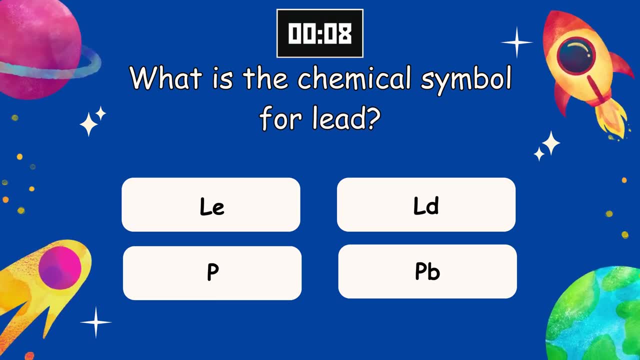 Correct answer is 24. What is the chemical symbol for lead? 10,, 15,, 16,, 17,, 18,, 19,, 20,, 21,, 22,, 23,, 24,, 25,, 26,, 27,, 28,, 29,, 30,, 31,, 32,, 33,, 34,, 35,, 36,, 36,, 37,, 38,, 39. 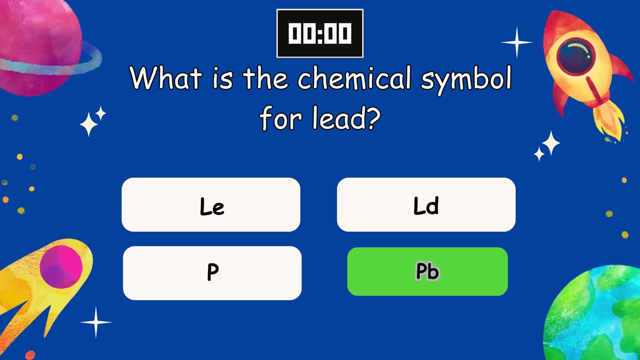 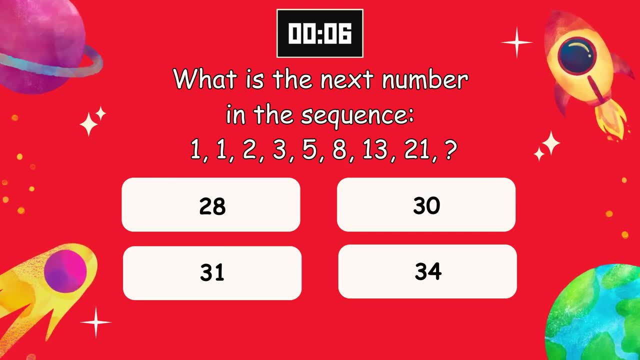 Key word question: What is the smallest prime number greater than 10? 3,, 2,, 0,, 4, 1? Correct answer is 12. What is the smallest prime number greater than 10? Three, five, eight, thirteen, twenty-one. 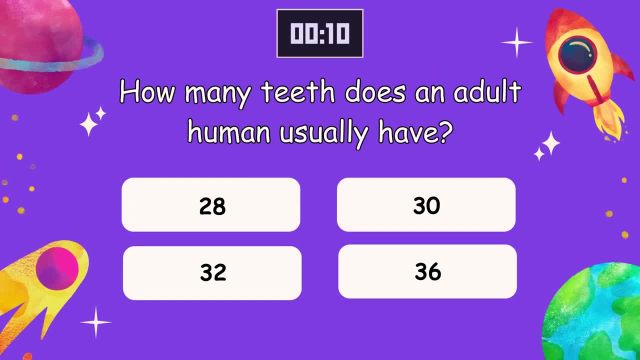 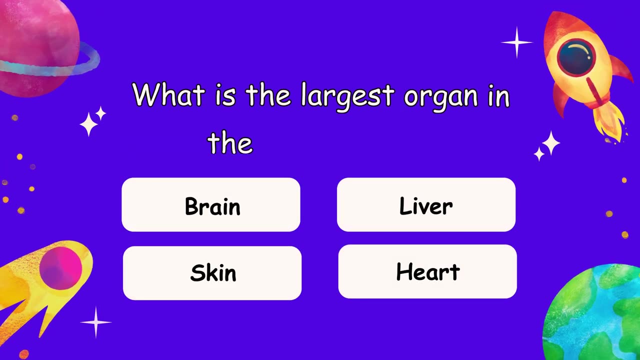 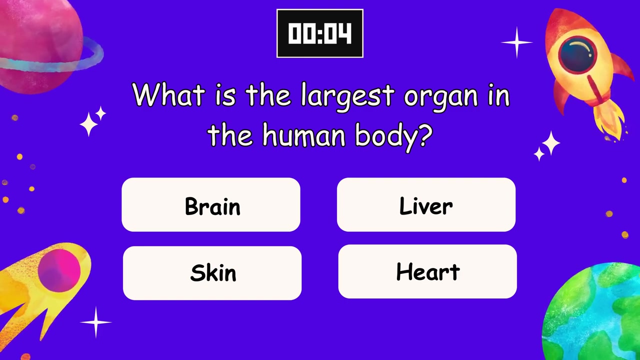 Correct answer is thirty-four. How many teeth does an adult human usually have? Twenty-eight, thirty, thirty-two, thirty-six. Correct answer is thirty-two. What is the largest organ in the human body? Brain, liver, skin, heart. 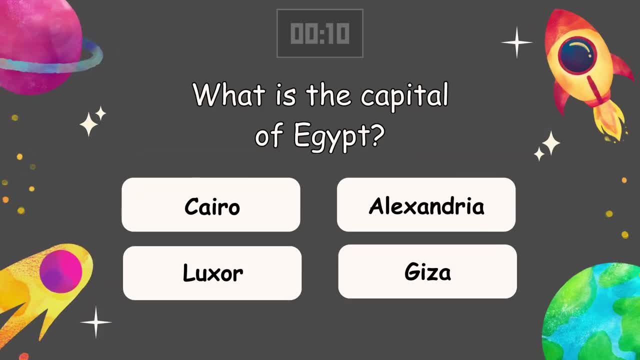 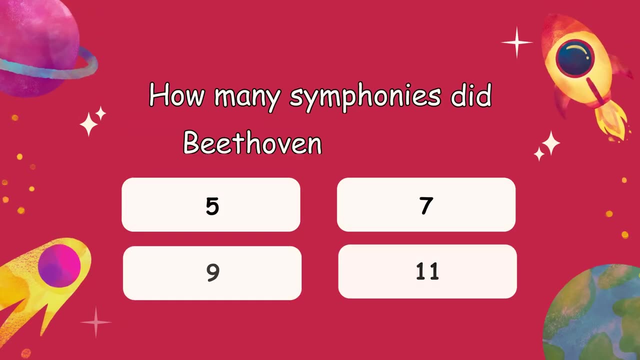 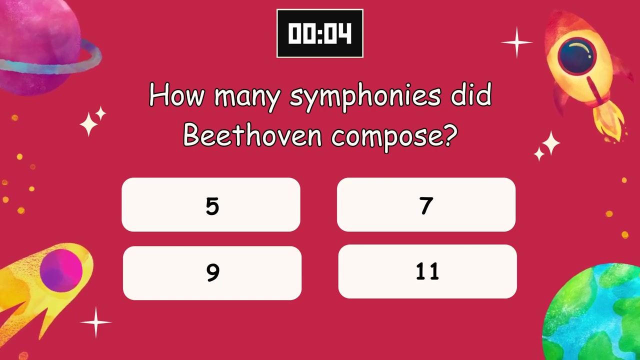 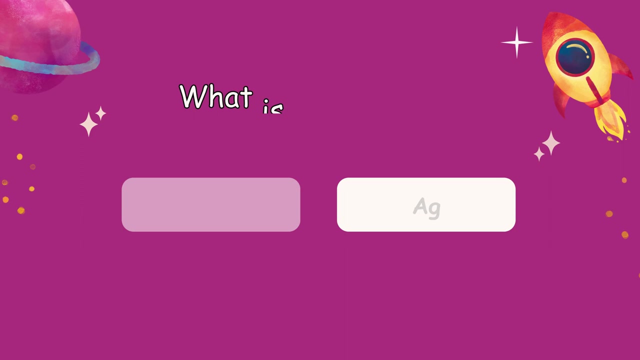 Correct answer is skin. What is the capital of Egypt? Cairo, Alexandria, Luxor, Giza? Correct answer is Cairo. How many symphonies did Beethoven compose? Five, Seven, nine, eleven? Correct answer is nine. What is the chemical symbol for silver? 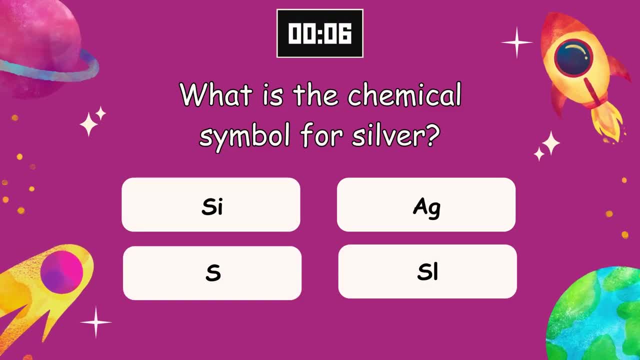 C, A-G, S, S-L. Correct answer is A-G. What is the next number in the sequence Two, three, five, seven, eleven? Correct answer is A-G. What is the next number in the sequence Two, three, five, seven, eleven? 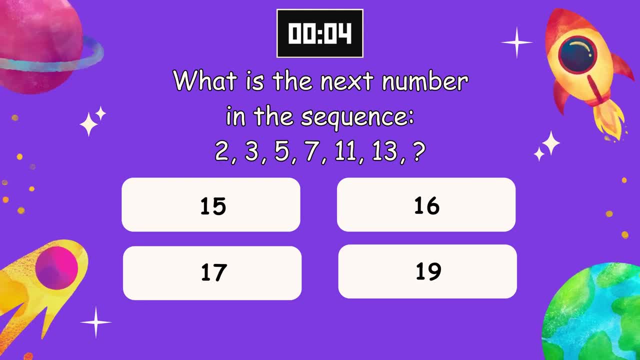 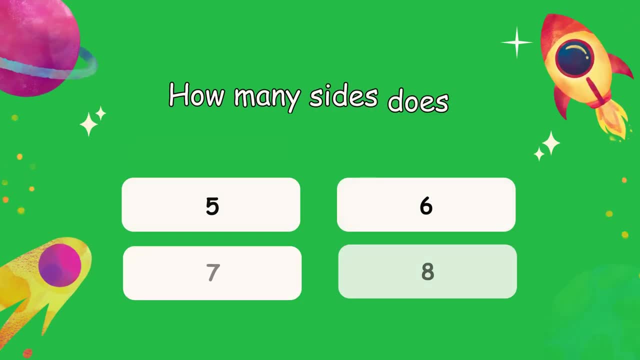 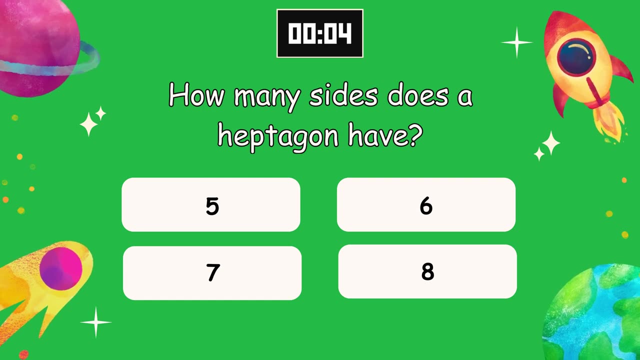 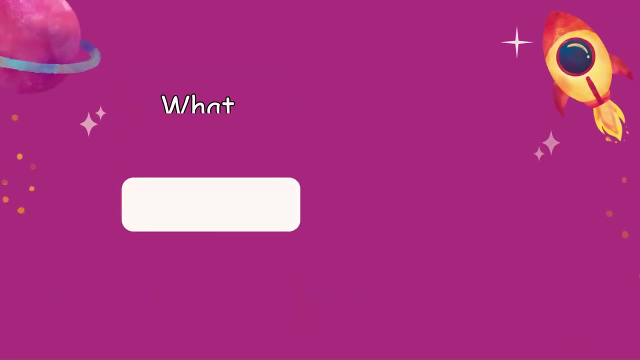 What is the next number in the sequence? Eleven, thirteen, fifteen, sixteen, seventeen, nineteen? Correct answer is seventeen. How many sides does a heptagon have? Five, six, seven, eight? Correct answer is seven. What is the opposite of expand? 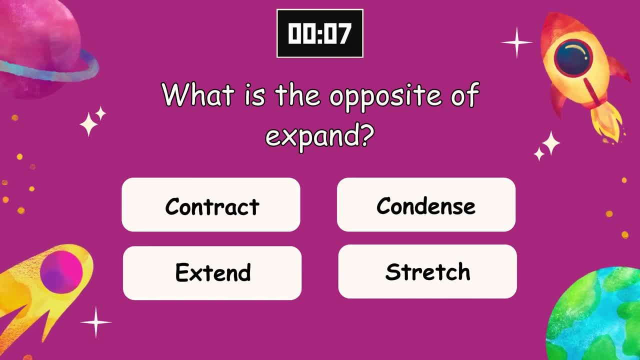 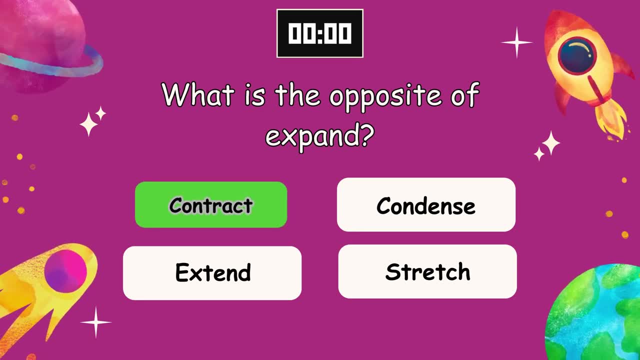 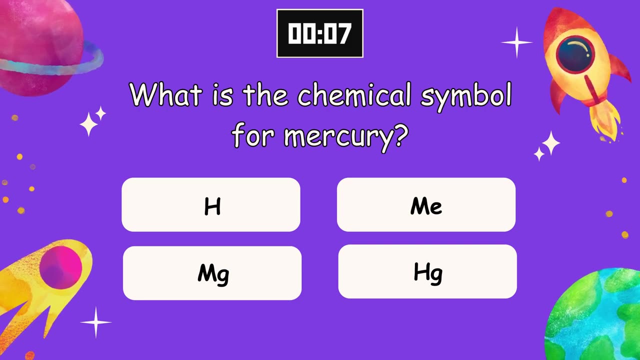 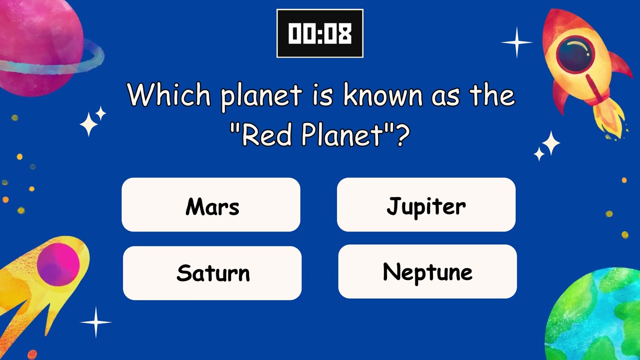 Contract. condense: extend: Correct answer is contract. Extend Stretch: Correct answer is Contract. What is the chemical symbol for Mercury? H, Me, Mg, Hg. Correct answer is Hg. Which planet is known as the Red Planet? Mars, Jupiter, Saturn, Neptune. 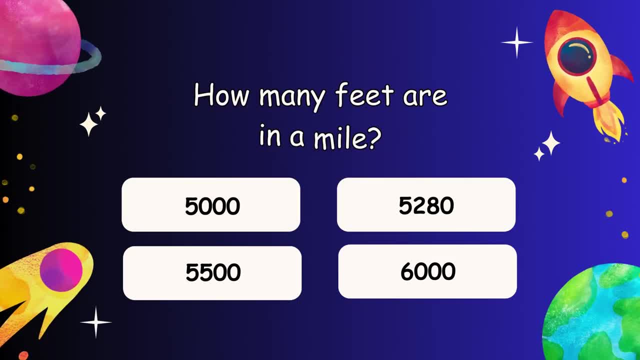 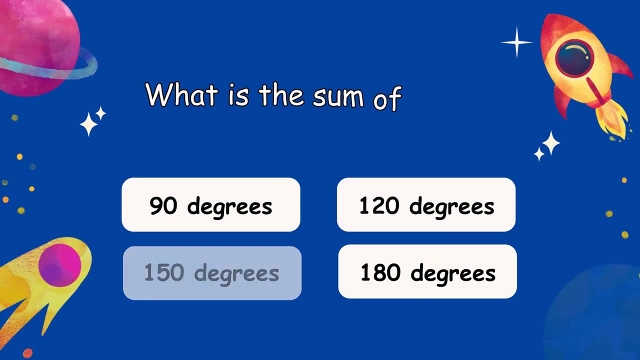 Correct answer is Mars. How many feet are in a mile? Five thousand Five thousand two hundred and eighty. Five thousand five hundred Six thousand. Correct answer is five thousand two hundred and eighty. What is the sum of all the angles in a triangle? Ninety degrees? 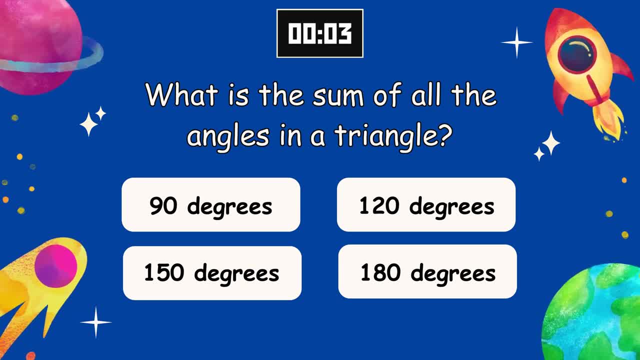 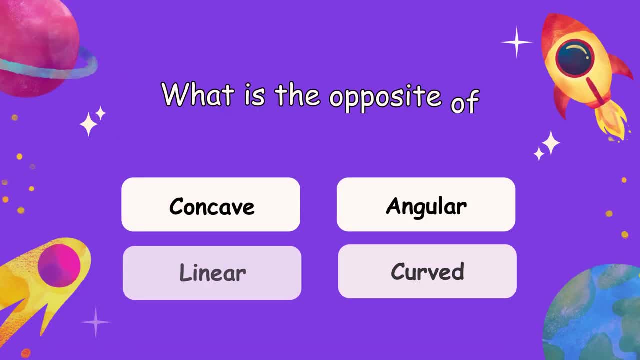 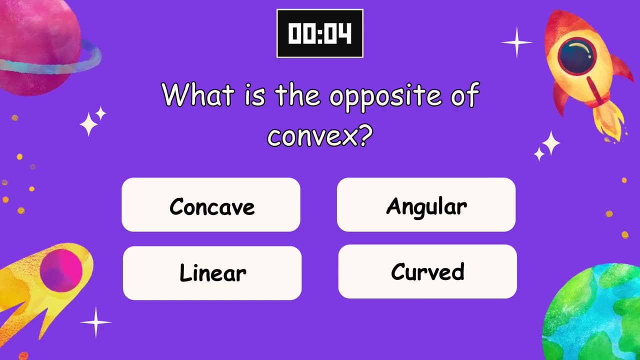 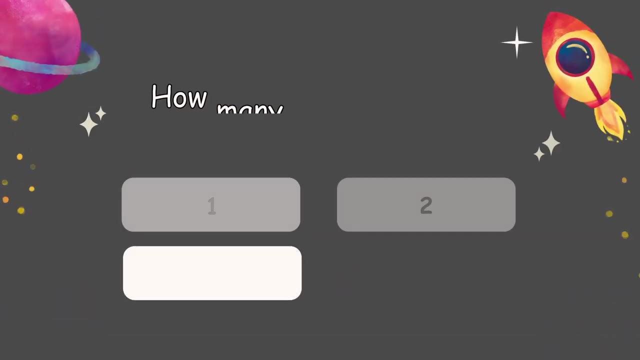 One hundred and thirty, One hundred and twenty degrees. One hundred and fifty degrees. One hundred and eighty degrees. Correct answer is one hundred and eighty degrees. What is the opposite of convex? Concave, Angular, Linear, Curved? Correct answer is concave. How many hearts does an octopus have?